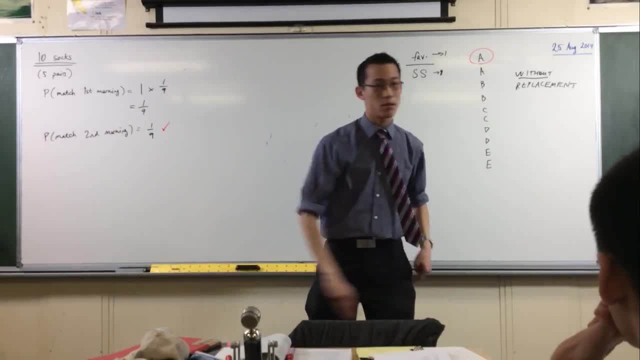 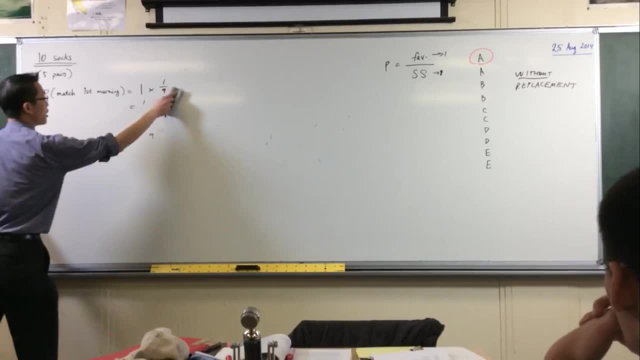 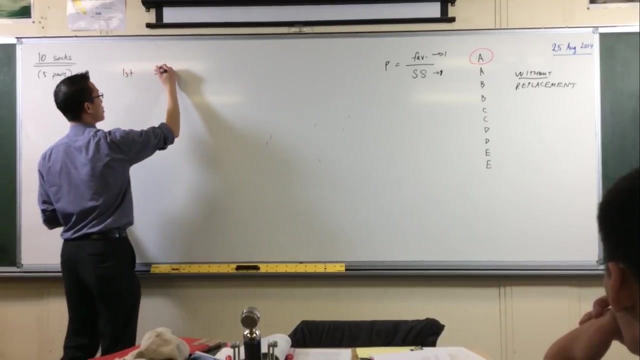 going to think about them, not just as mornings. I'm going to think about those individual socks. Okay. So I need- I need more space, We'll do this, And you're going to need more space too. So rule off. whatever you're doing, I'm going to have a first sock. Whoops A. 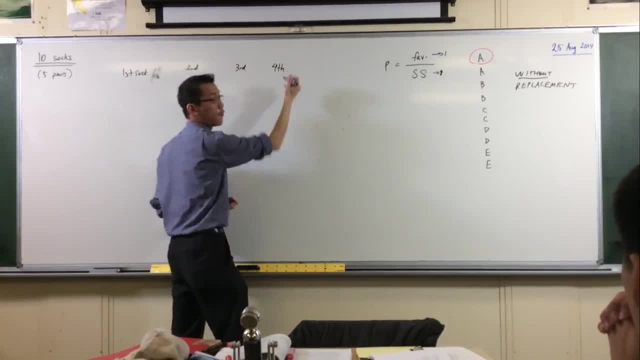 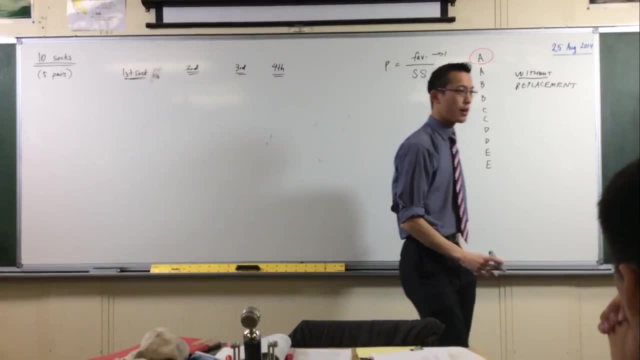 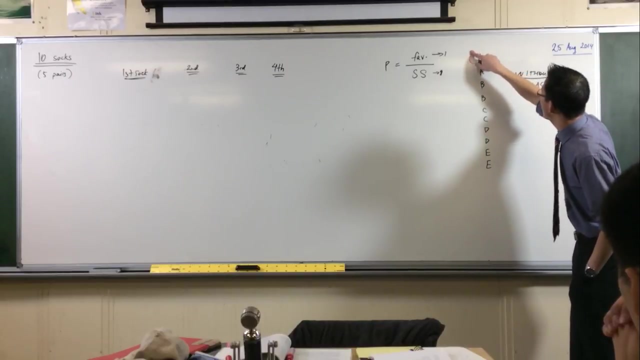 second, a third and then a fourth. Okay, So this is what I'm going to go through. Let's rehearse again from scratch. Okay, For the first sock that I pick, here are my choices. Okay, Sorry, I haven't picked any yet. Okay, So does it matter which one I choose? Still, 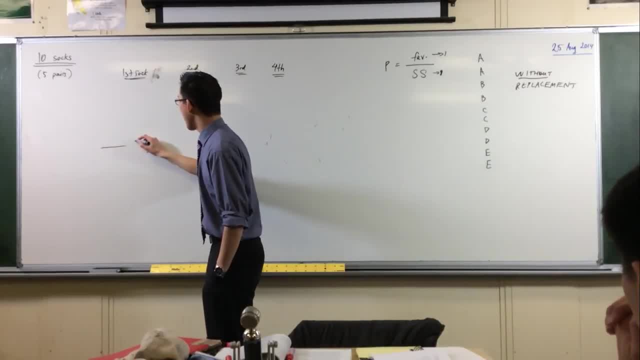 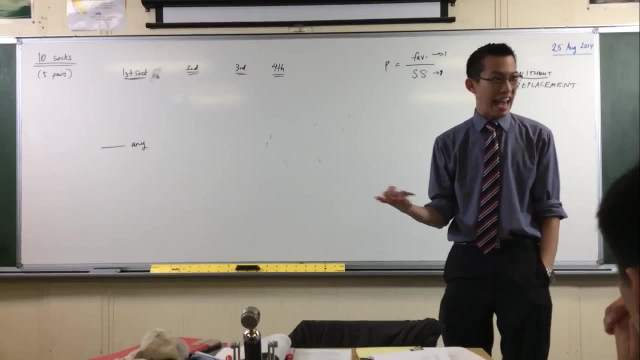 doesn't matter, does it? Okay? So here's my first sock, Right? So I can actually pick any sock. That is the only probability that I'm interested in Right Now. if I were to draw this out like: actually I've got 10 to choose from, but I don't want to have a probability. 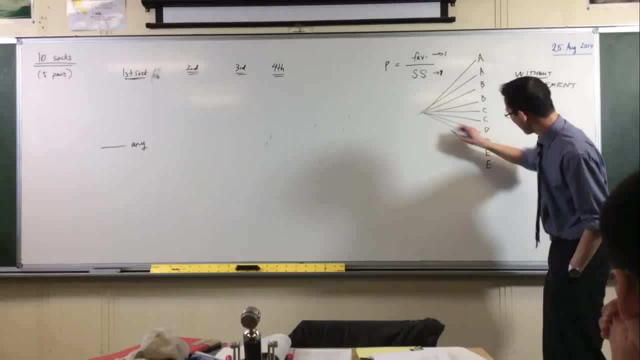 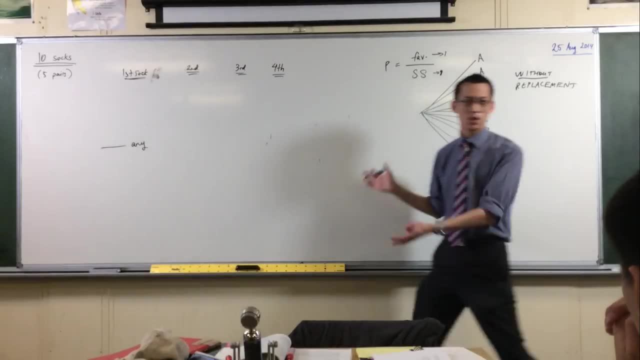 of 5,, 6,, 7,, 8,, 9,, 10 branches, Because even with one level, let alone 2,, 3, and 4 levels, it's already unworkable. Okay, So I'm going to condense it down. What's the probability? 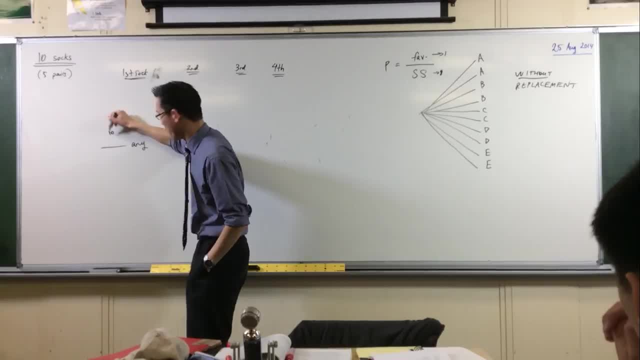 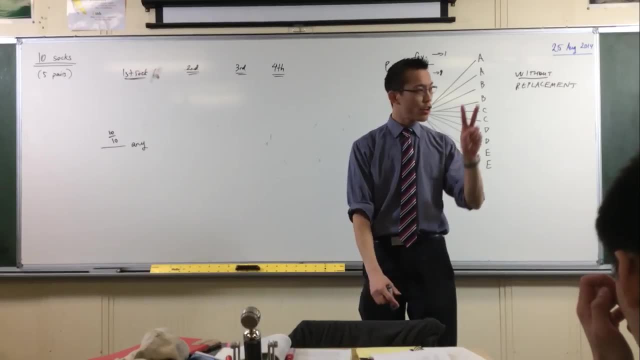 of picking any sock. Well, just like before, there are 10 favorable outcomes and there are 10 total outcomes. So far, so good. Great. Now I go to pick out the second sock. Okay, Here there are two alternatives, and we need to consider them differently. 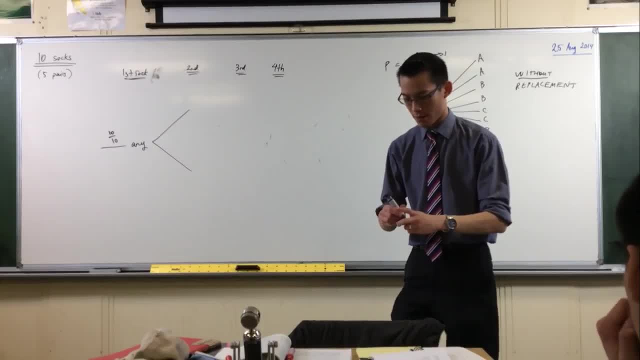 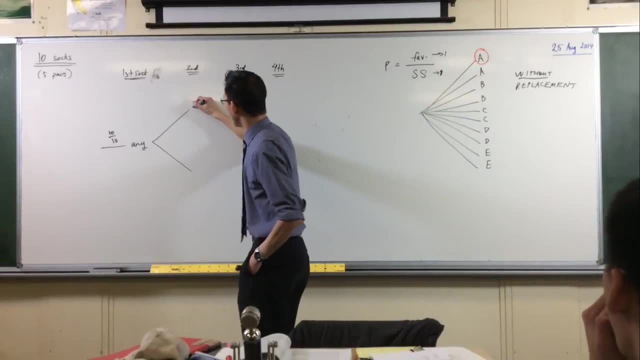 I hope you'll see why in a second I'm either going to pick- sorry, so I've picked a sock now, so I'll circle this again- I'm either going to pick a sock that matches that one. it'll be the same. 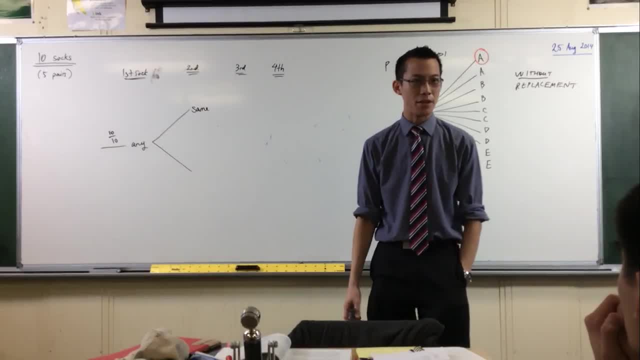 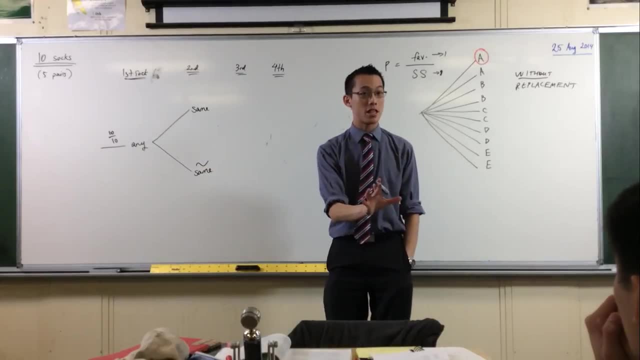 or I won't. It'll be different, So not the same. We've already worked out this part of the question. This is going to be 1 over 9.. Notice the sample space. by the way, Can you see why I didn't just write 1?? 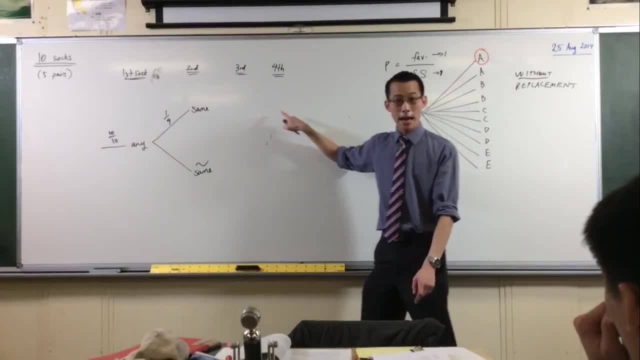 I want to see. this will be 10,, this will be 9,. this is going to be out of 8,, this is going to be out of 7.. Build it in a way that makes the logic easier to see, not harder. 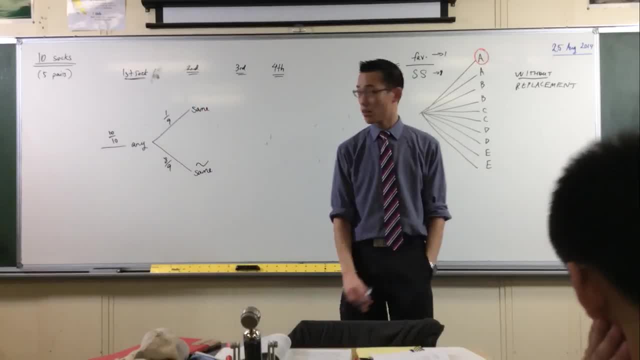 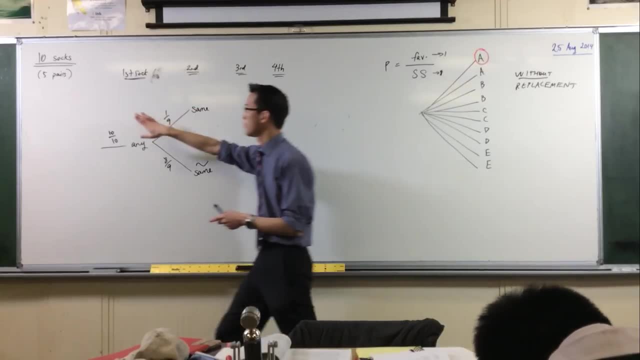 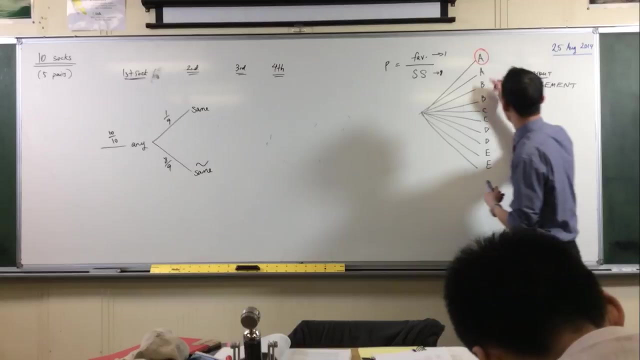 That makes the complement 8 over 9.. So far, so good. Now let's think about here: If I picked this, is now this scenario. I picked a pair that matches That's this morning here, So that was this one. 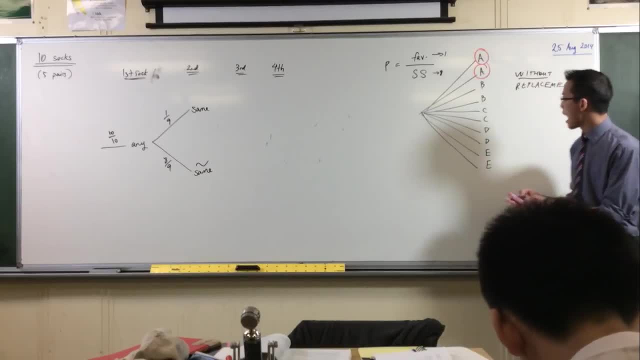 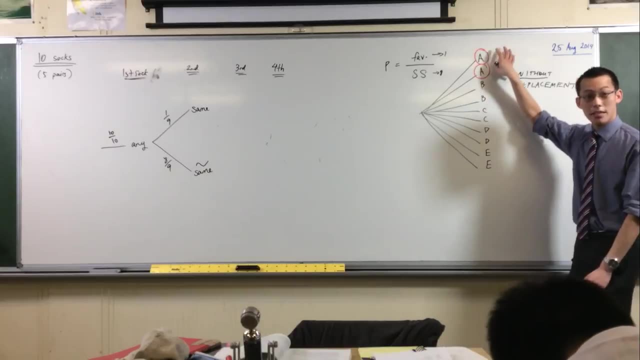 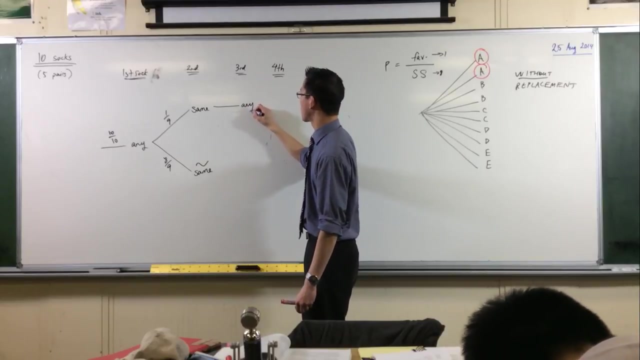 Let's think about this now. I have 8 choices. Does it matter which of these 8 that I picked for my third sock? It doesn't matter, I'm in exactly the same situation I was in the first morning, So therefore, going here, I can pick any sock that I like. 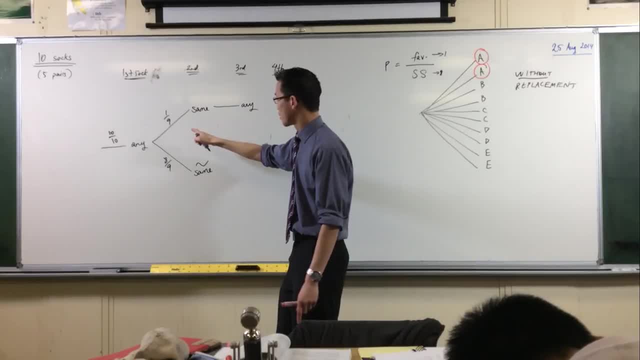 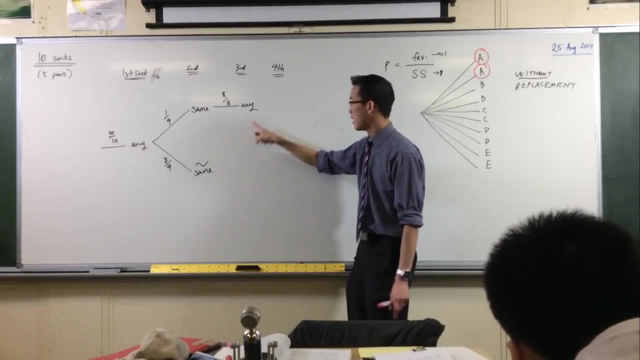 provided. I picked a match the first time, So this went 10, 9,. this will be 8 out of 8.. Is that okay? I'll come back to this one. Let's complete what happens here, because it's easier. 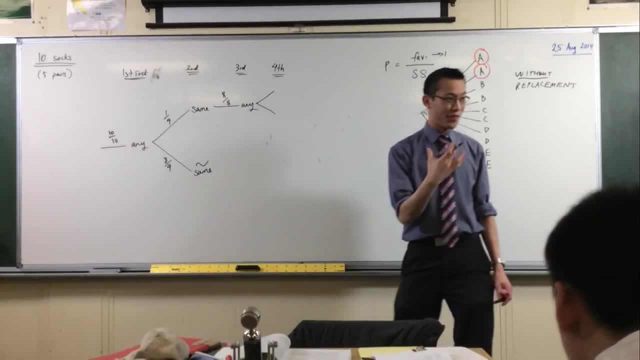 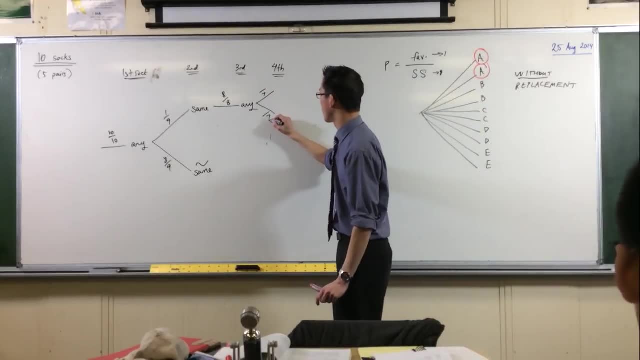 Now, just like the first morning, I'm in the same scenario. How many socks are left? Well, it's going to be out of 7.. I'm either going to pick a fourth sock that matches the third, or a fourth sock that doesn't match the third. 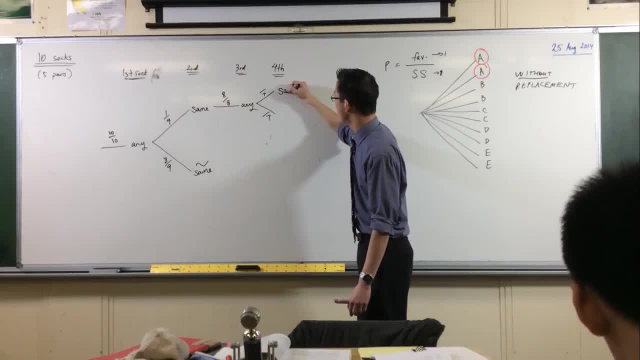 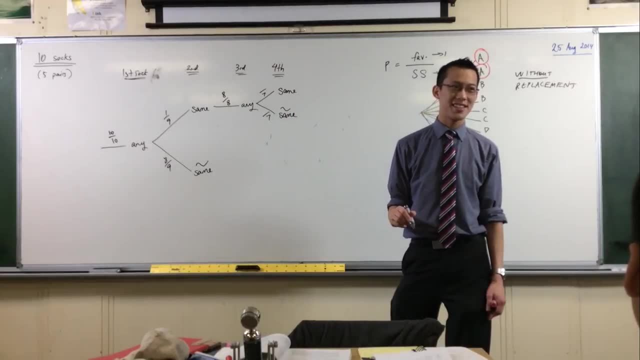 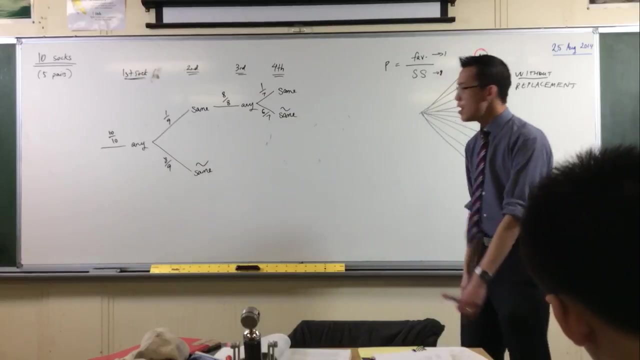 I'll be in this scenario again: Same or not same. Are you happy with that idea? How many socks are the same as the one? I picked One, And then you got the compliment. Okay, excellent. Now let's come down to this guy, right? 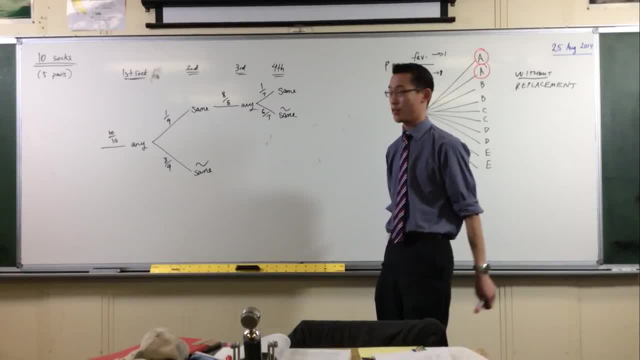 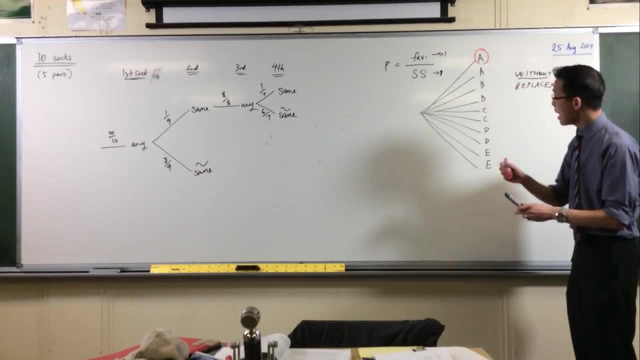 The game changes and this is why it's so important to have the probability tree. I didn't pick socks that are the same right, So I didn't pick A and A. I picked, for example, A and B. Okay, pause. 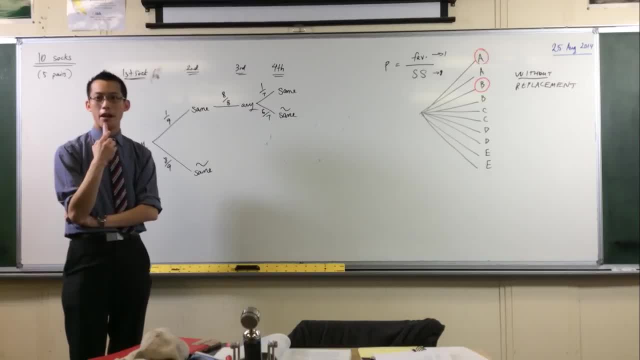 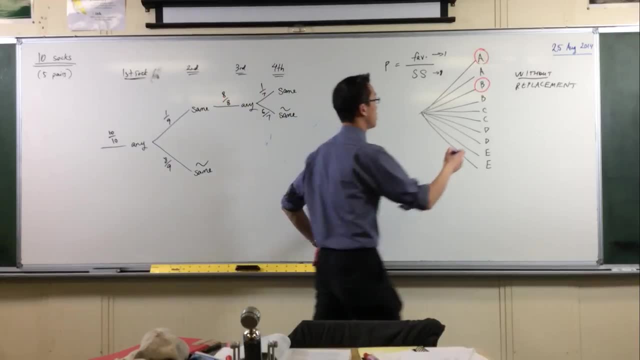 Does it matter which of the 8 remaining socks that I pick? And the answer is: it does matter. It does matter, It makes a difference. okay, Because if I pick my third sock to be A, I'm stuffed already, right. 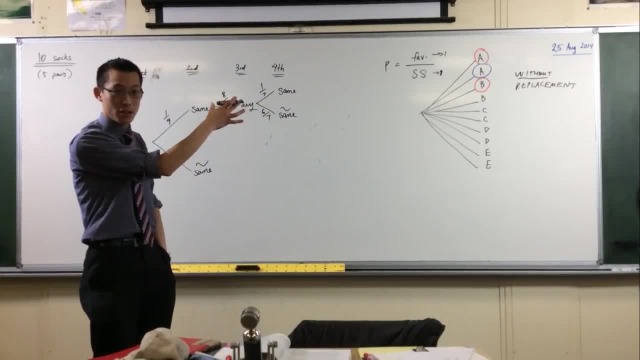 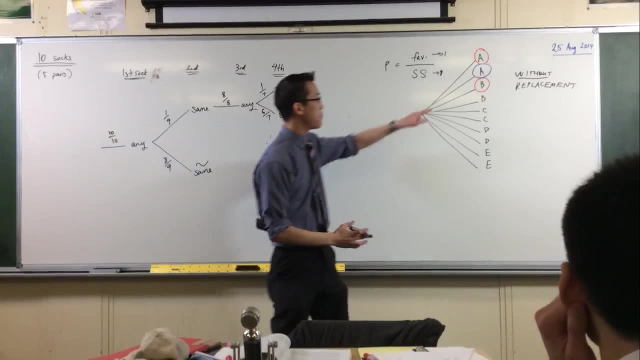 There's no chance, having picked A on the second morning, because I already got A out of the drawer yesterday. as Elian says, it was in the wash okay, So there's a zero chance. if I pick this guy, it's impossible that I'll get a match. 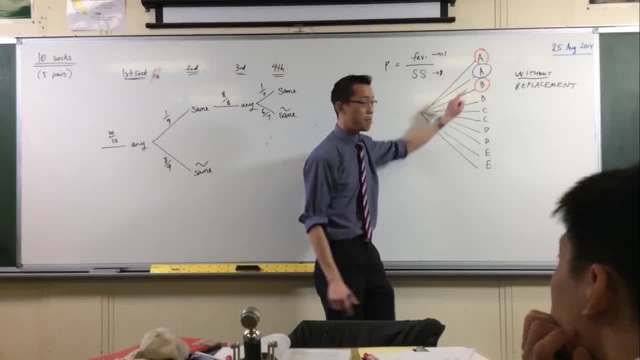 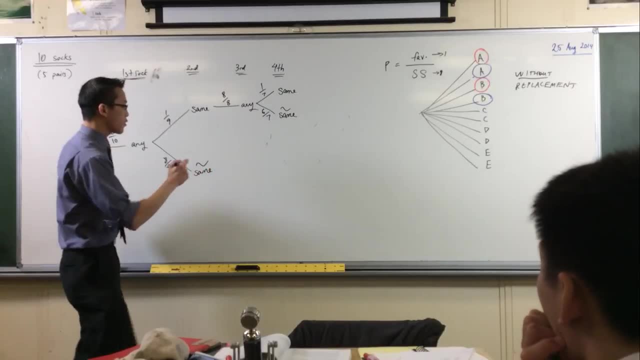 A is not the only one, which is the other one, B. If I pick B, I'm similarly up the creek. I'm going to have to hide my socks all day. okay, So therefore there is two possibilities here, right? 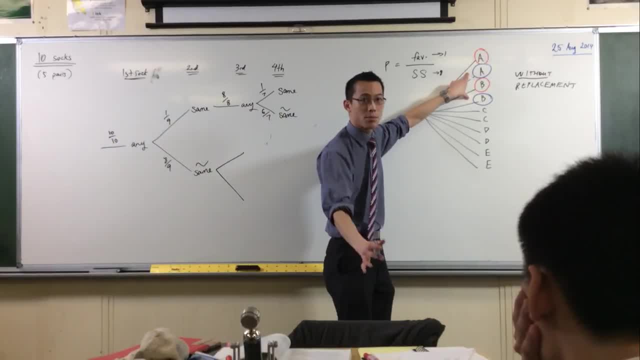 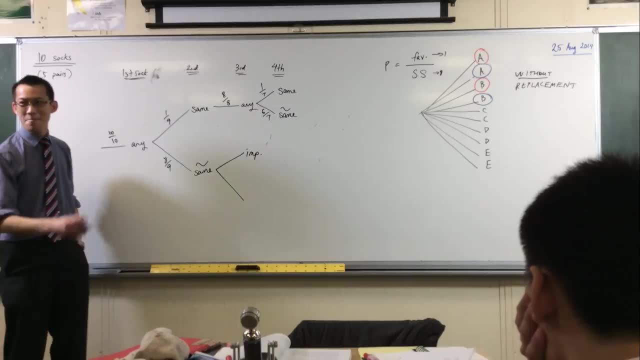 I can pick a sock that makes it impossible to get a match. okay, So I'm going to call that very Doctor Who. I'm going to call this the impossible sock. okay, There's a sock I can choose which gives me no chance of getting a match, right. 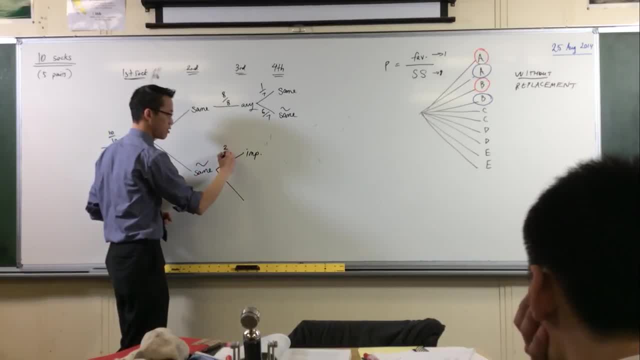 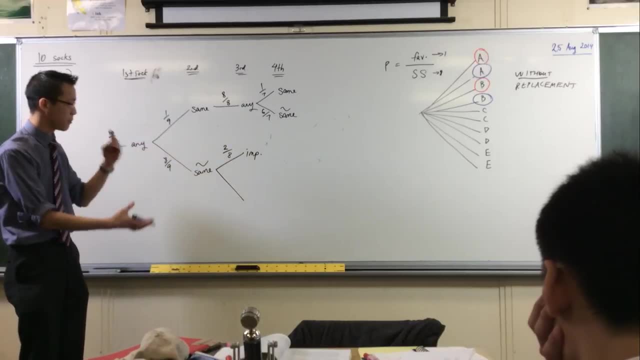 And there are two of them out of eight. okay, Two out of eight. Of course you can write a quarter there, But can you see why I'm not right? I'm trying to make the sample space clear. So therefore you know, obviously. 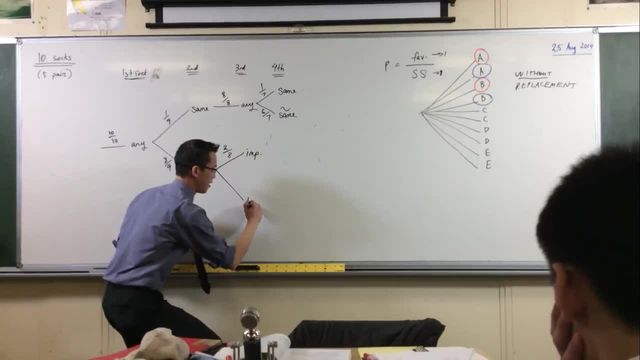 I could write the complement of impossible. that's a bit of a double negative, so I'm going to write there. you know I can pick a sock. that does make it possible. I can still get a match. and because it's the complement, 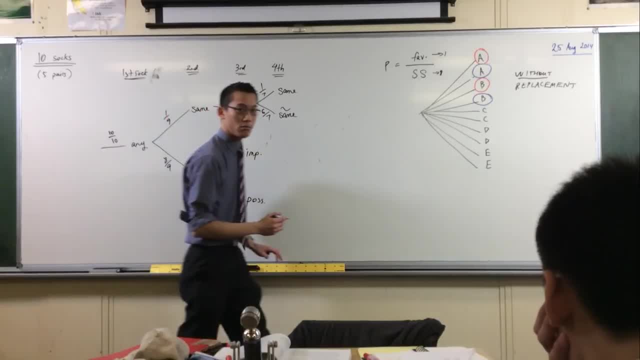 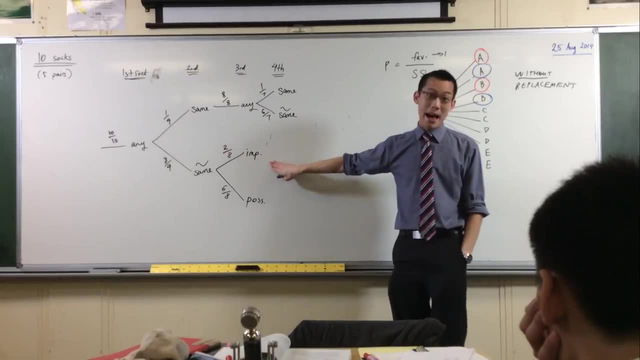 six out of eight. So far, so good. Good, I forget about this guy now. I'm not interested in him because all I want- I rubbed it off, all I want is a match for the second morning, so I don't worry about him anymore. 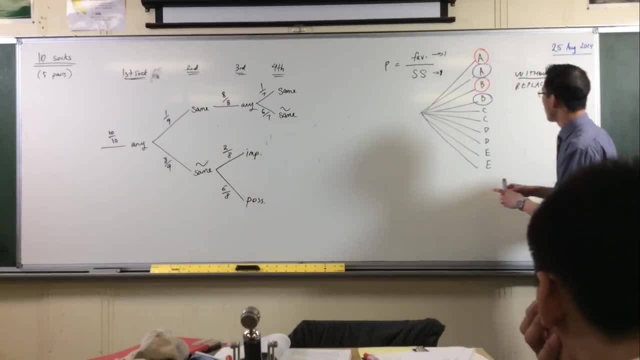 I come down to this one, right. So I didn't pick one of these impossible socks, right? I've now picked out. for instance, I picked out C, That's a possible sock, isn't it Okay? And then I've got two possibilities. 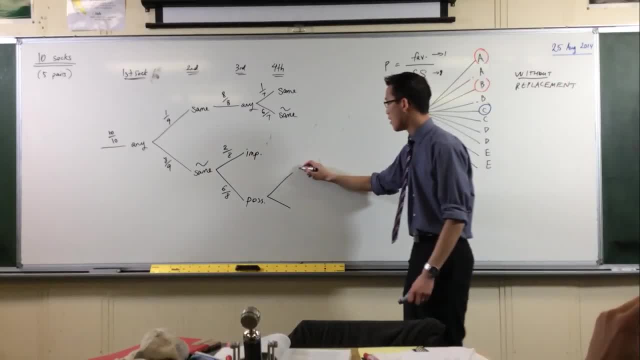 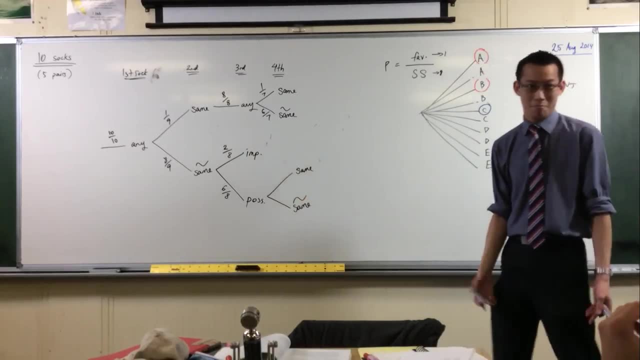 I'm going to get a match or a not. I'll either get one that's the same or not the same. Okay, What's the sample space? Well, there were ten socks here, and then nine, and then eight. 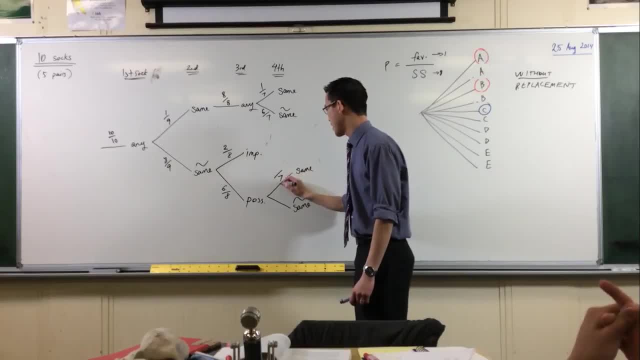 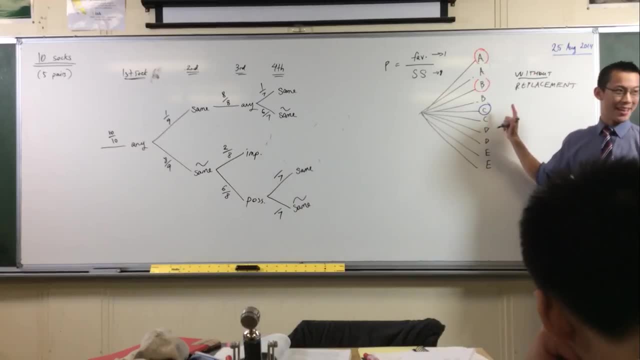 and then seven, right, So this is going to be out of seven out of seven, because I've already pulled three out. I picked C, Colour C. How many socks are the same? One, And then the other six are different. 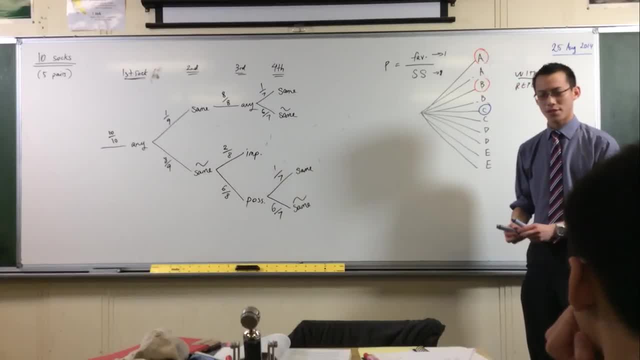 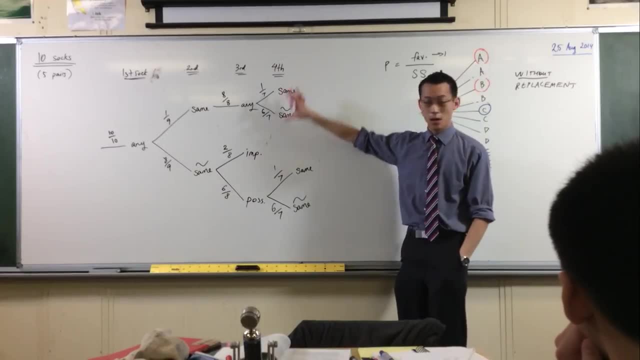 Okay, Now what was the question I was after? I was trying to work out what's the probability of getting a match at this point. Okay, So that's this one. That's this branch here and this branch here, Right. 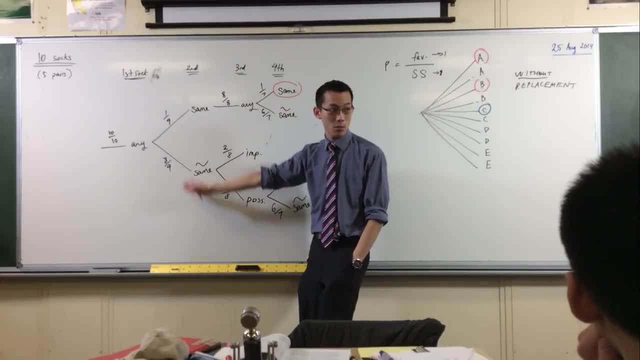 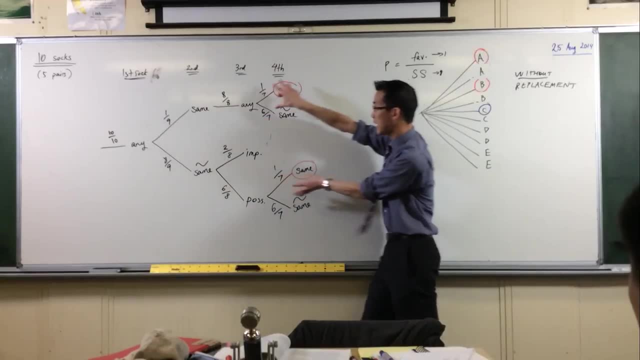 Those are the ones where I have a match on the second morning and I don't really care what happened on the first morning. Okay, So let's work out each one in turn and then we can add them together. Product rule to get to here. 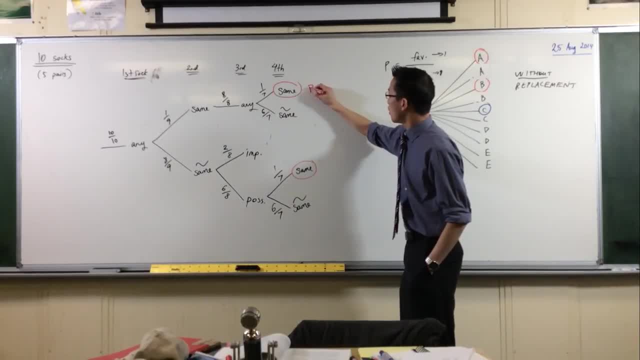 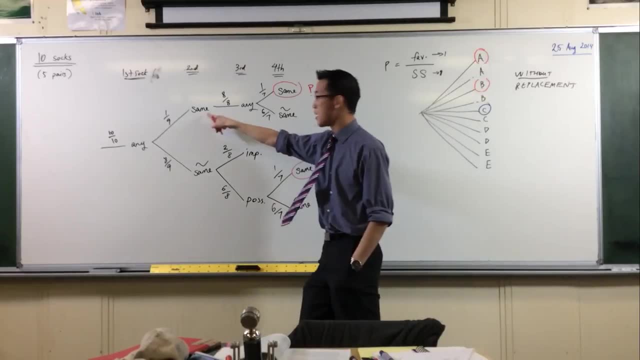 additional rule to put these guys together, Okay. So what would I call this one? I'd call it: same same Two mornings, Same both times, Okay. So the probability of getting it same twice right is one times a ninth. 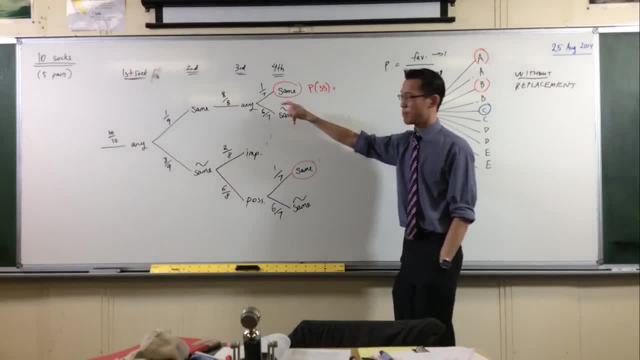 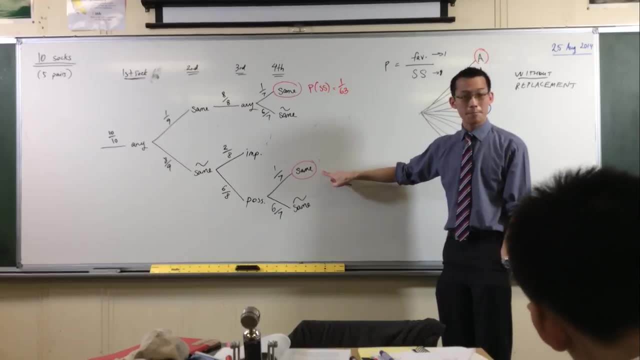 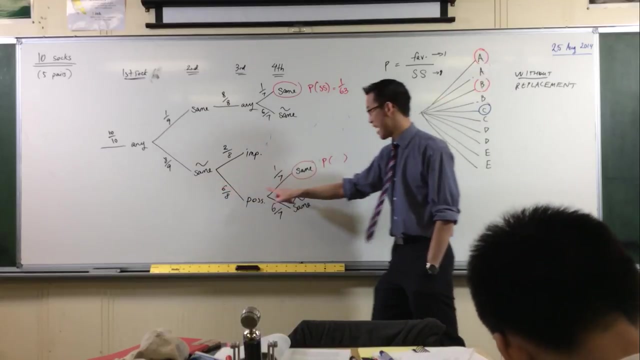 times one times a seventh. Is that okay? One on 63.. Seven times nine. Yeah, Now I have a look at this one. What should I call it? I guess I would call it not same and then same. 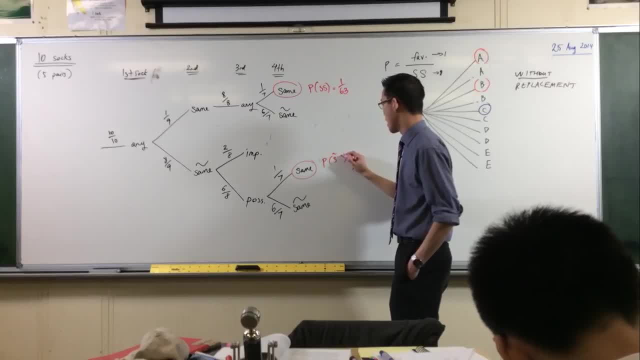 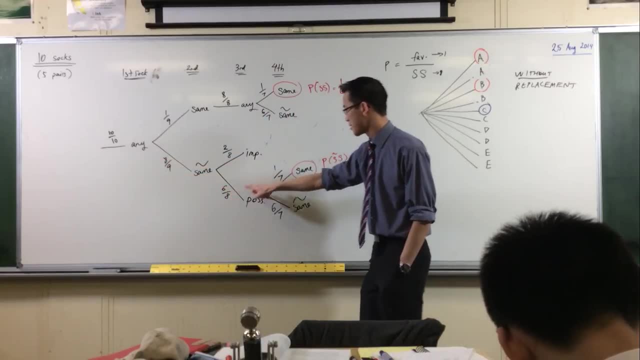 That's what happens each morning, So not same and then same. The probability is going to be one times eight, ninths times six, eighths times one, seventh, Four events right, And they're all strung together. 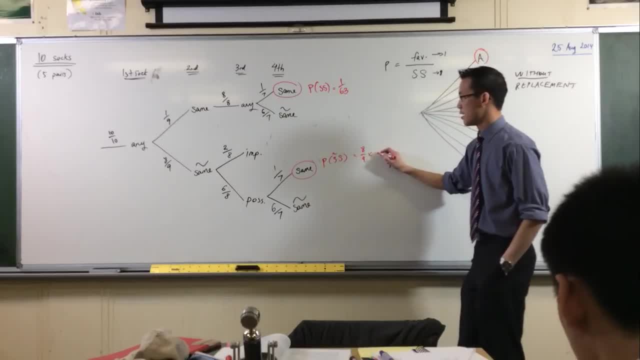 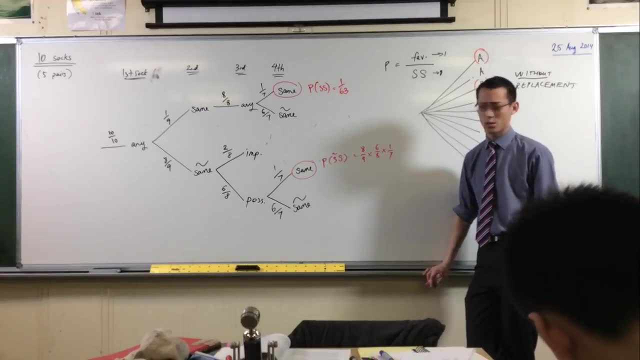 I won't worry about the one. I've got eight over nine times six over eight times one over seven. I've got some fractured business here. I can cancel some stuff here. I can cancel some eighths. Right, I get left with six on 63.. 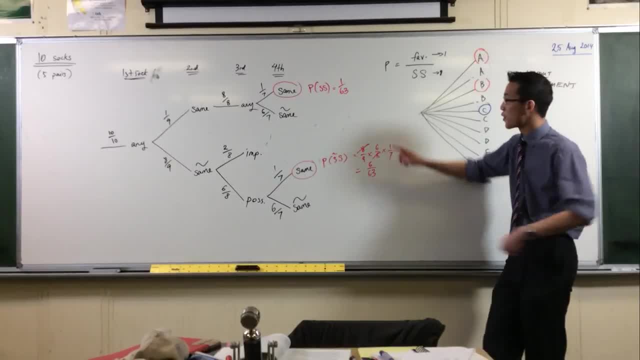 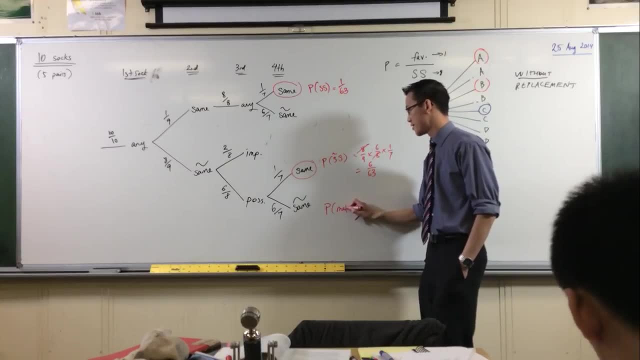 Of course I could simplify that further, but I'm not going to Because I want to add these two. Right, These are my two possibilities. I should add them. The probability of a match the second morning. it looks to me like it's one on 63,. 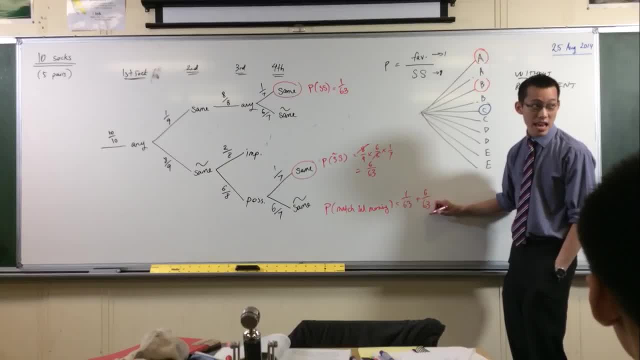 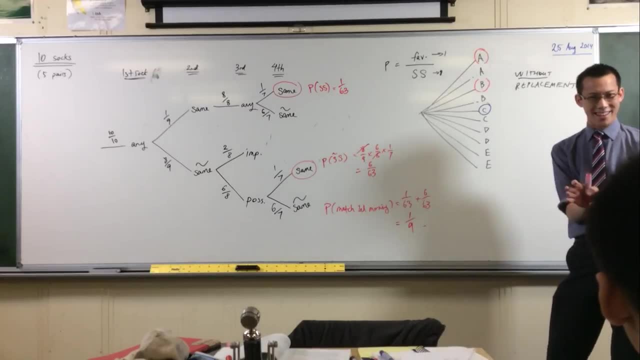 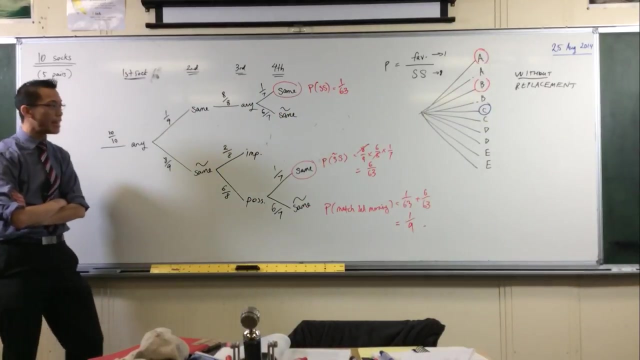 plus six on 63.. That's seven on 63, which is a nine. So hold on a second. What just happened? Okay, We confirmed our original answer. Sure enough, it's a nine. Okay, But it's weird. 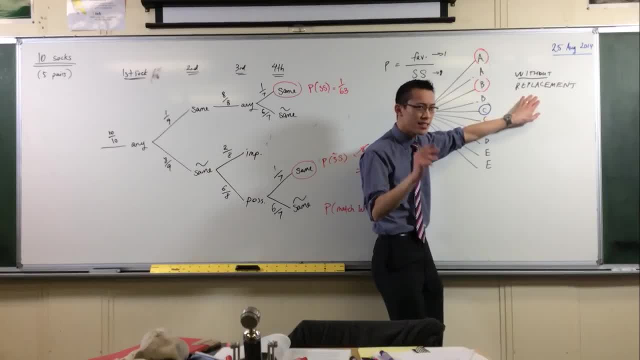 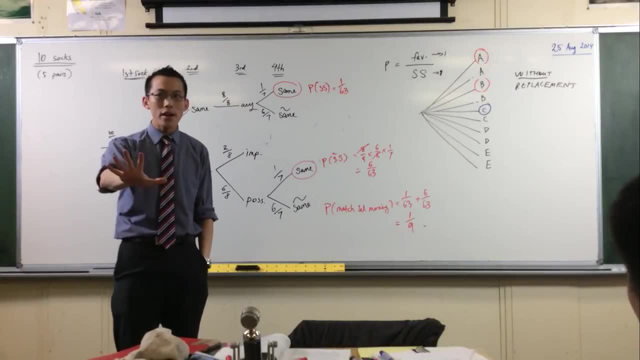 There's no replacement going on. It doesn't suggest that you would get the same probability of a match the second morning as you would the first and the third and the fourth and the fifth- Always the same. Okay, I think the reason why is because